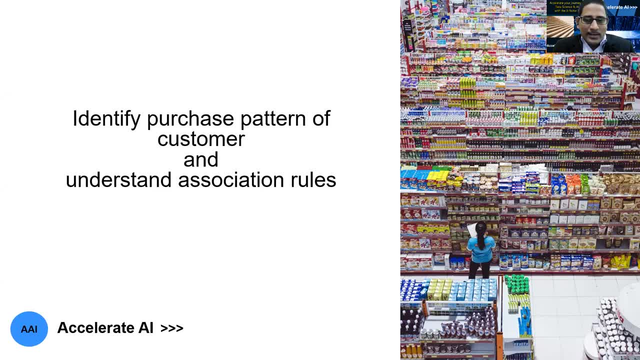 and buy those two inadvertently. You might seem to think you made a decision to buy those and it was solely on you. However, the placing of objects in the aisles is done in a strategic way and it encourages you to explore the store until you have bought more than what you need. 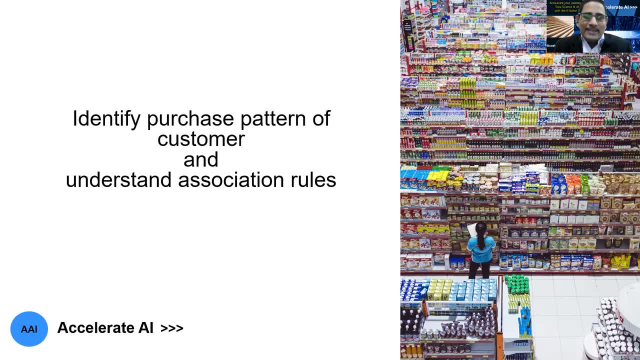 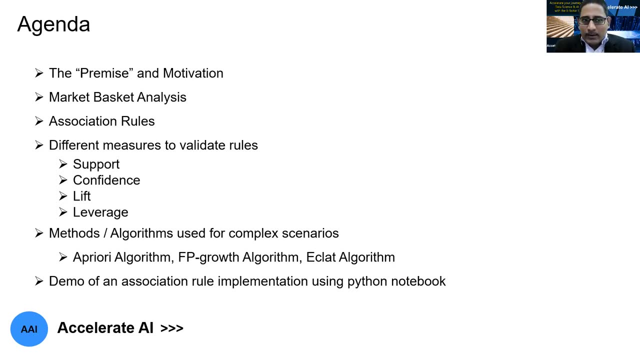 So let's understand how this is happening And this is a classic example of market basket analysis, Kind of association rules which we call, and we'll talk about that. So, as part of today's agenda, we'll be focusing on quickly on the premise and the motivation. 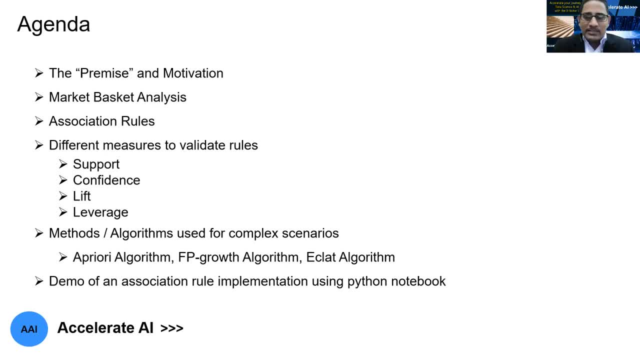 of unsupervised machine learning and how does it help into these kind of problems that we face in business? Then we will talk about the market basket analysis. We understand the association rules, then different measures to validate those rules and how they work, And then we'll talk about the market basket analysis. 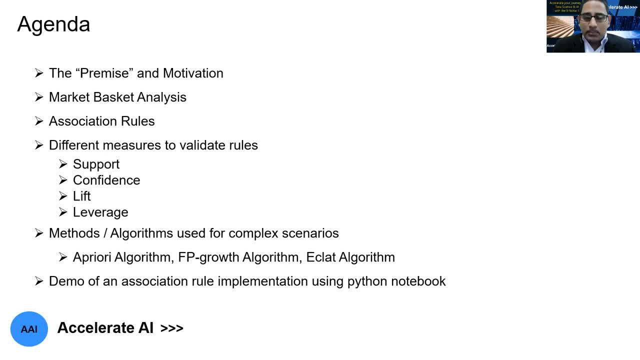 Then we'll talk about the market basket analysis. We understand the association rules. there are certain measures such as support, confidence lift and leverage. We'll talk about those. Then we'll talk a little bit about methods and algorithms used for complex scenarios. 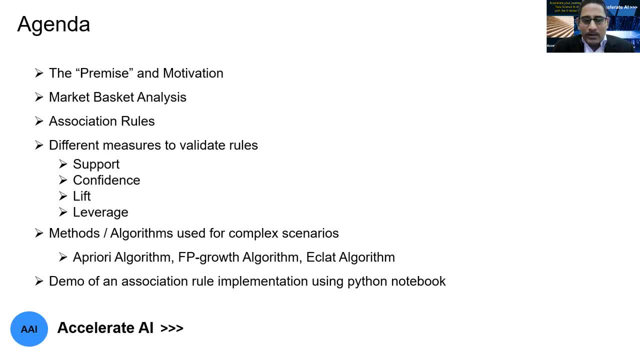 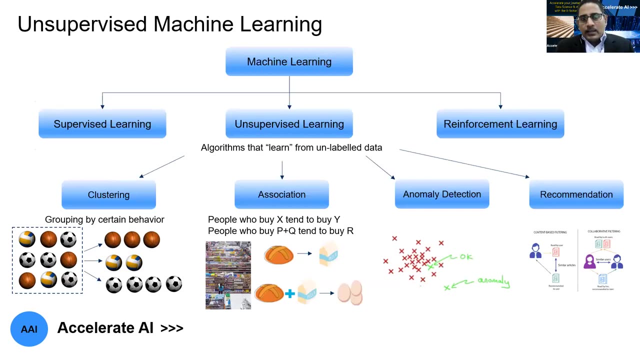 A priori. algorithm is one of the key algorithms, and we'll talk about that, And then, of course, we'll latch on to a quick demo of an association rule implementation using a Python notebook, Before you look into unsupervised machine learning. Now, this is something which is 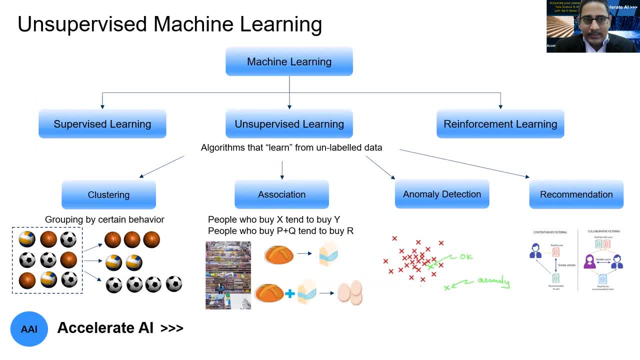 where algorithms that learn from unleveled data right. We have supervised unsupervised and reinforcement learning, The unsupervised one, where the algorithms learn from the unleveled data. There are different techniques as part of it. One could be clustering, association, anomaly detection. 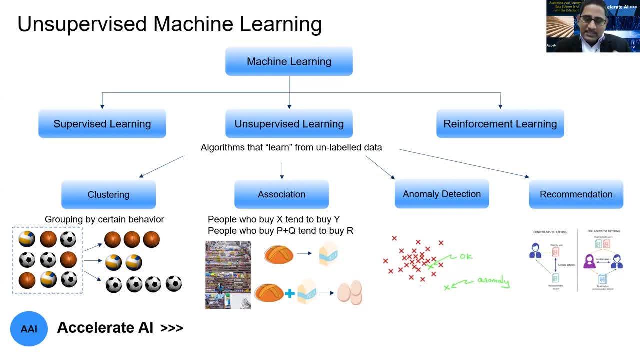 recommendation and so on. There are different techniques as part of it. One could be clustering, association, anomaly detection, recommendation and so on. If we look at specifically, let's say, clustering, you're trying to group certain behavior and try to categorize them, whereas when you look into 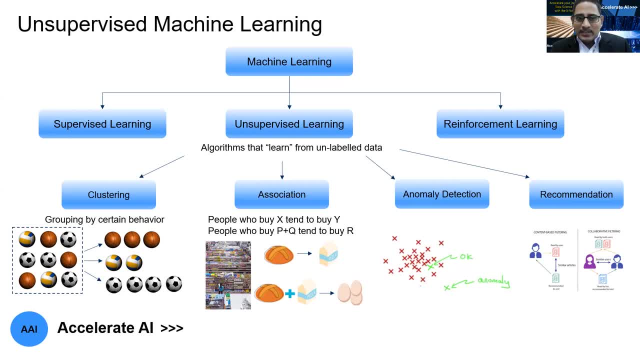 association, the scenario is different. You're trying to identify people who buy X, they tend to buy Y. People who buy P plus Q, they tend to buy R. So that's what we are trying to kind of understand, And this is important here as well. 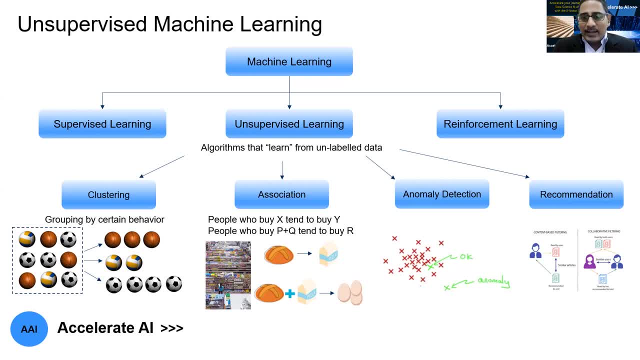 people who buy x, they tend to buy y. people who buy p plus q, they tend to buy r. so that's what we are trying to kind of understand. So that's what we are trying to kind of understand part of it, and that's where association will come into picture. let's take an example you'd have 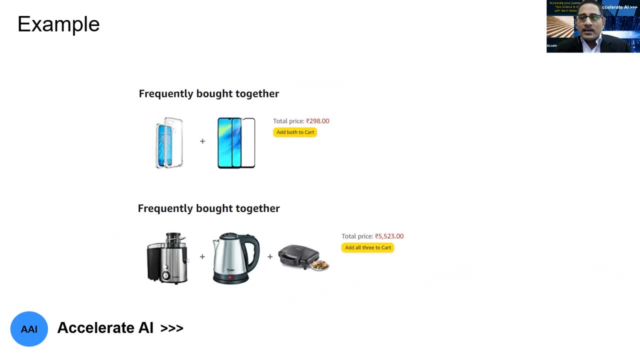 noticed these recommendations while making your purchases right. some of the examples of these are very practical in nature when we look at it, and if you, if you talk about something like a mobile cover, then obviously it is prompted with the added, you know cover of some of these that 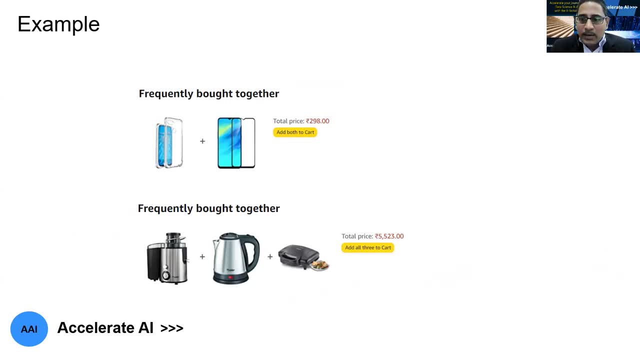 that have been frequently bought together. if we are talking about a coffee maker, then you know the the sandwich maker along with the juice maker. is this going to be proposed or recommended? so that's typically what we have seen right. so that that's. that's an example which we can correlate. 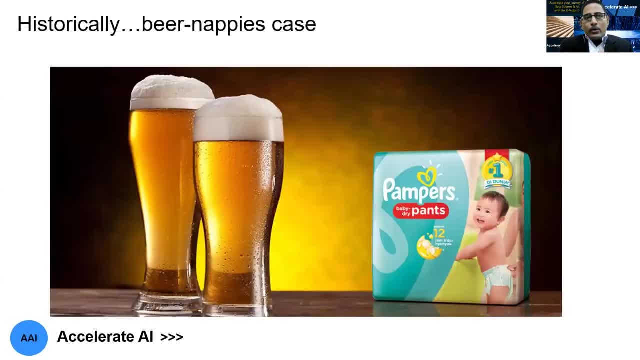 to association. Similarly, if we go historically, you know the famous example of beer nappies case. the story of correlation between the beer and diaper sales is very, very common to to explain the product affinities in in data science. Now what has happened is the analysis of 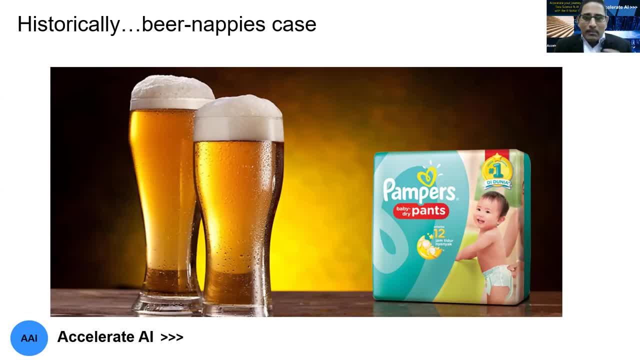 some of these purchases revealed that they were made by men, typically in the weekends, around Friday evenings. So basically, you know the beans were其實 própria nutritious beans. 투 is matching the male and female size of the beans, Several cases from six pm to seven pm and the retail stores where it was found. they 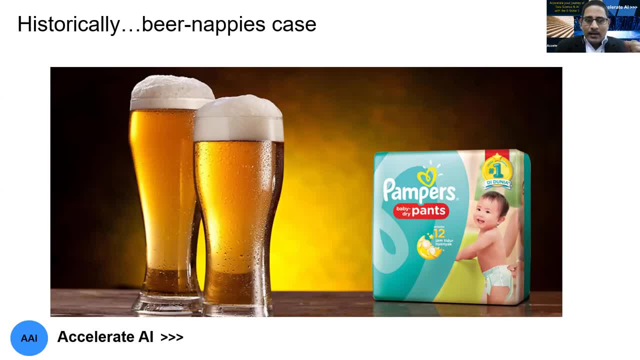 have found some very specific rationale behind it. one: since the packs of diapers were relatively large in size, The wife, when most cases made the household purchases, left the diaper purchase to the husband for their babies, so probably they have gone and picked it up. That could be one ration. 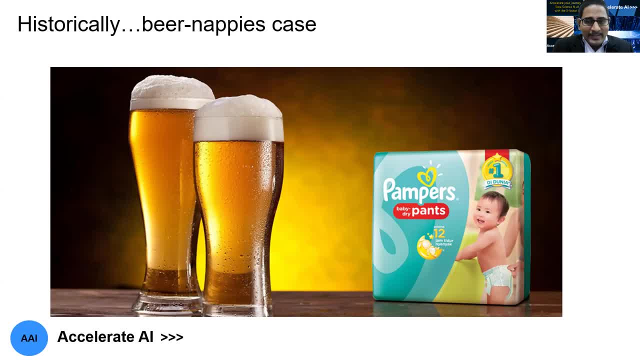 Second being the end of the working week, the husband, historically early in his family, maybe in the late 90s, had already bought a range surface and lost that small piece of the piece of the of against, I'll built a unleash harvest bye. and then the father also wanted to get some beer in for the weekend. um, you know, that's probably the. 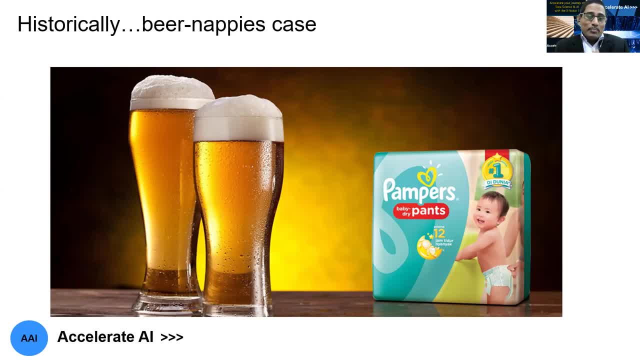 background of it. but what? what they did that they put the premium beer display next to the diapers. so it's kind of an upsell, right. so you're upselling your other product, which is which can be correlated. the result was that father's buying the diapers, who also usually bought beer, as it was. so 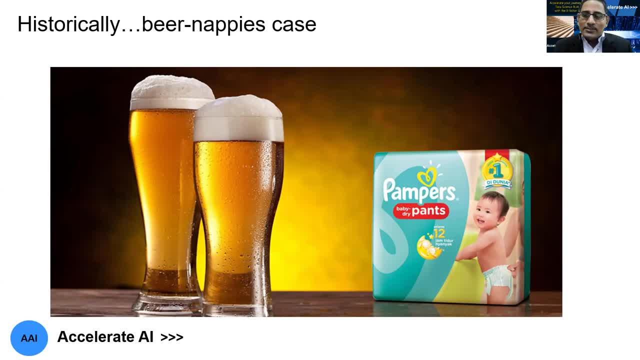 conveniently placed next to the diapers so that you know the upsell happens more in a seamless manner. significantly, when we look at, men did not buy beer before began to purchase it because it was so visible and handy just next to the nappies. so it's kind of a cross sell as an example. so net. 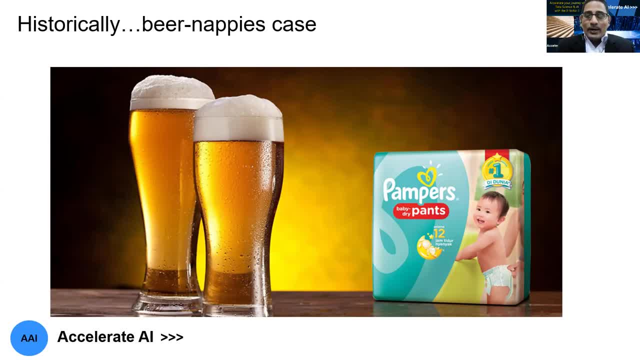 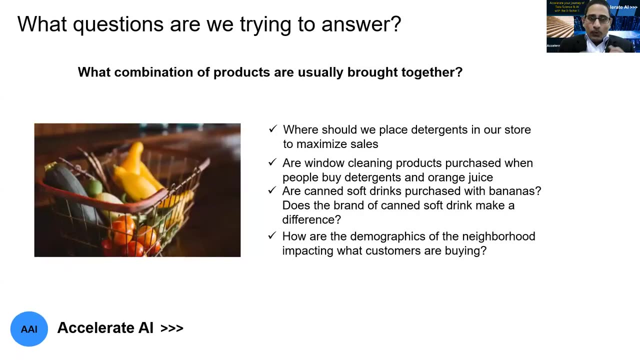 result is as beer sales skyrocketed. so this is a classic example of how historically this this has happened, and an example of the the association, and that's where the market basket analysis is an example. this is what it is, so what questions are we trying to answer as part of this right we? we try to look into what 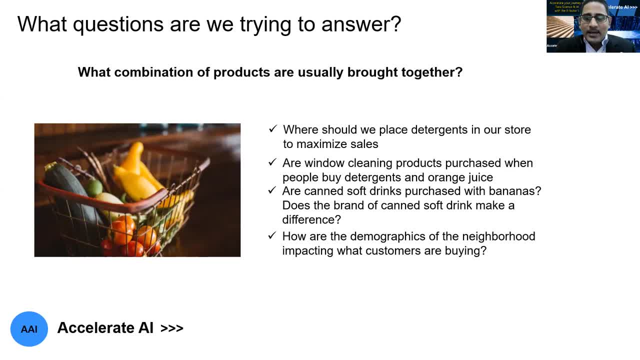 combination of products that are usually brought together, right? so you look at some examples like where? where should we place the detergents in our store to maximise the sales right? are the window cleaning products purchased when people buy diaper detergents and orange juice? if, if that's a kind of analysis that we are getting in, then then we 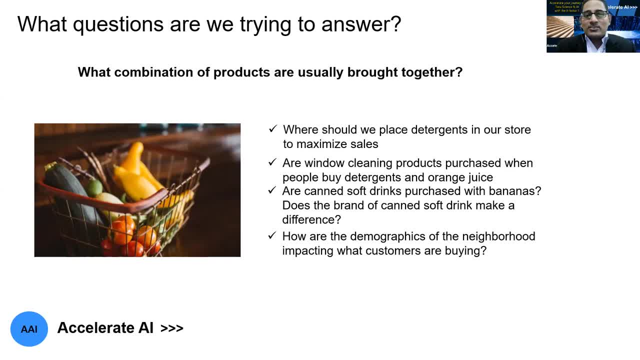 can actionize our steps accordingly. as a store manager, store owner, you know they can actionize it appropriately. another question of example could be: are the canned soft drinks purchased with bananas now does the brand of canned soft drink make a difference? then, accordingly, you know they can plan and actionize that way. how are the demographics of the neighborhood impacting the? 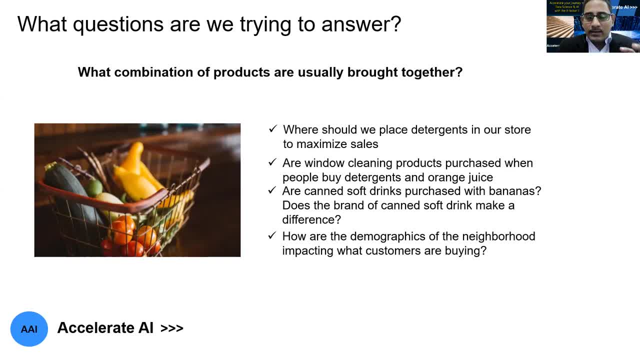 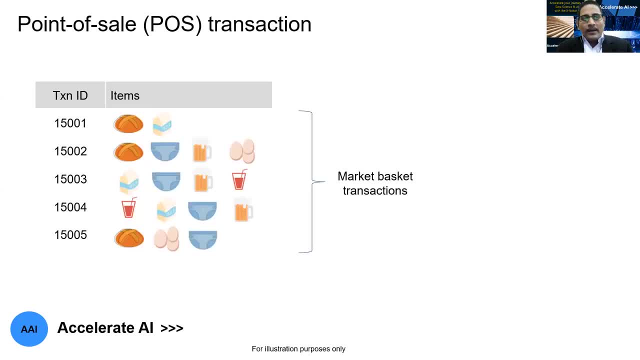 customers who are buying this right. so a lot of these questions. when we look at it, it looks into the combination of products, usually that part together, and which is what is the premise of it. now let's take an example. when we look into a point of sale transaction, which is in this case, 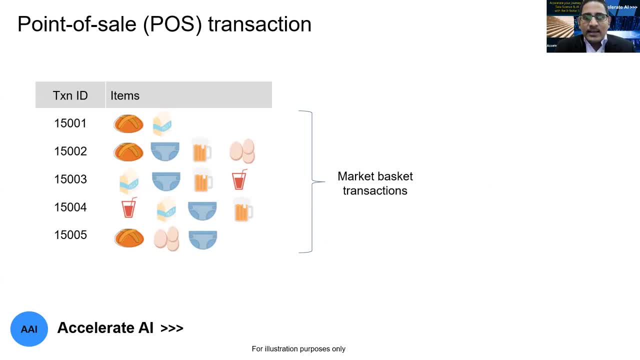 represented with five different transaction ids. these are all called market basket transactions, right? so let's say, the first transaction: you have bought the bread and milk. the second transaction: you have bought bread, the diaper, the beer and the eggs and so on. right, so this is an example of market basket. 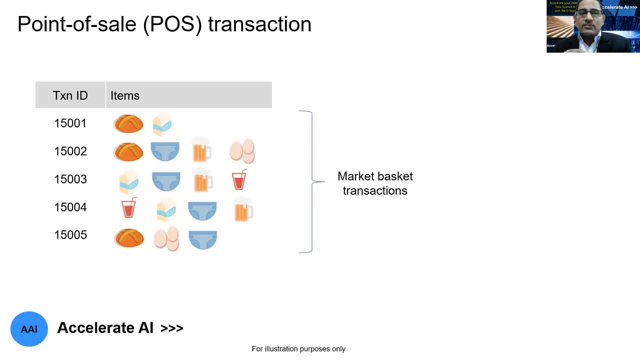 transactions, each having transaction ids, and a set of items that we kind of buy as part of it. you know which is what is captured here. as an example, now, what is a frequent item set? right, right, we can't really go with a brute force approach. frequent item sets is like why the combinations of 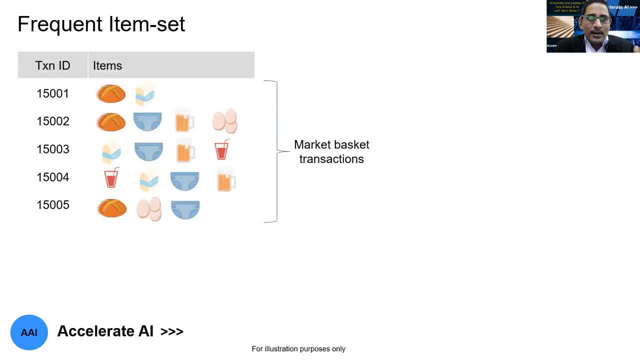 the items that are presented right, we'll have to start looking at it. what is happening here? so there, if you look at it, the frequent item set is nothing but the unique set of these. and then there are how many such unique items? six unit items if we look at in the set of five transactions. 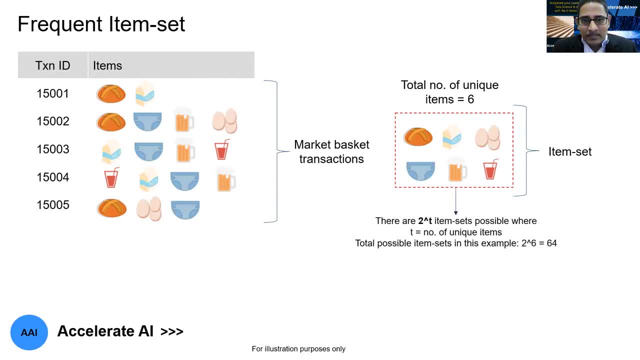 that we have considered as part of this example. now what's happening is that could be two to the power six or two to the power t item sets possible, where t is the number of unique items, so total possible item sets. here you could imagine two to the power six, which is 64, and that's a lot with just about six unit items when we consider as an. 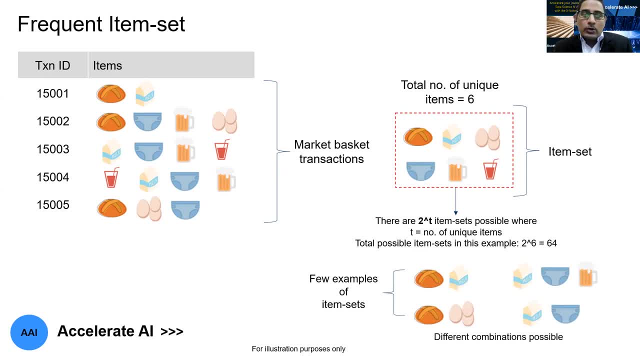 example, right now, few example of the item sets could be. you can consider bread along with milk, bread along with eggs, and then milk with diaper, with beer, then milk with diaper. there could be a lot of these different combinations possible, right, however, what we call a frequent item set. 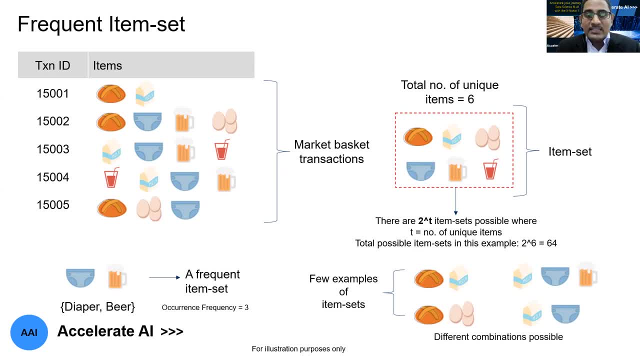 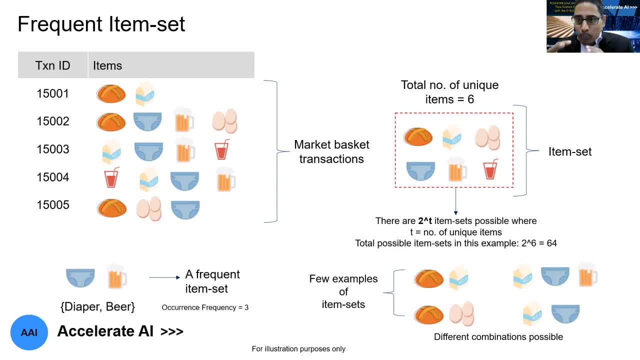 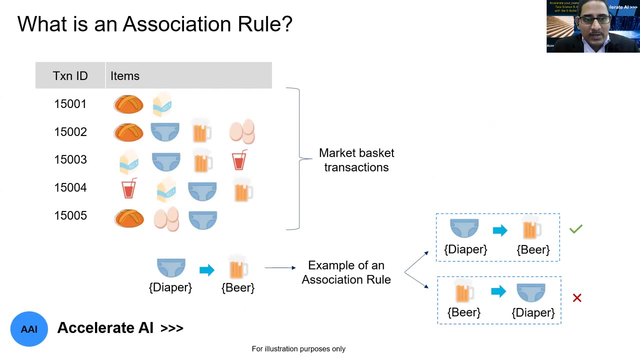 15004. so there are three occurrence of both together. that's the frequency, occurrence frequency. hence it is a frequent item set. now, looking at what is an association rule in the same example, when we look at this as a market basket transaction, then what we're trying to see here is: if beer, if diaper, then beer right. 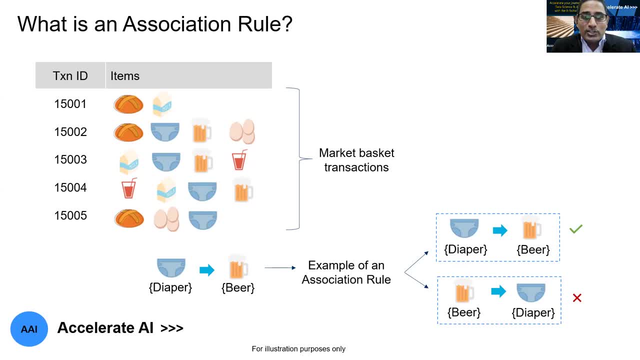 that's an example of a frequent item set. so if we look at this as a market basket transaction example of an association rule, if you are buying diaper, then you are buying beer. now emphasize here is on why the association right. why are we saying diaper? if diaper, then beer, why not? if beer, then 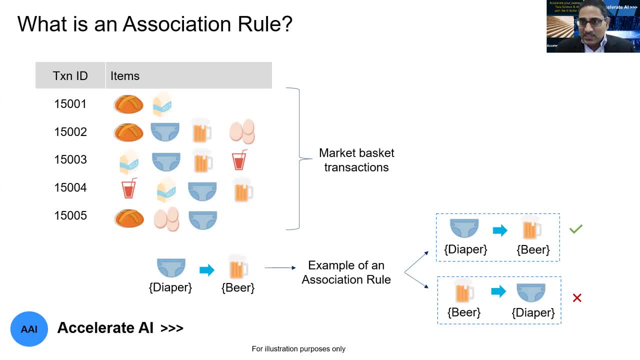 diaper, because if you look at, in this set of transaction set, wherever you have beer you have the diaper that is available, so it's it's all preceded by the association rule. so if you are buying diaper, then you are buying beer based on this transaction set, whereas here there is a diaper but there is no beer. so which means 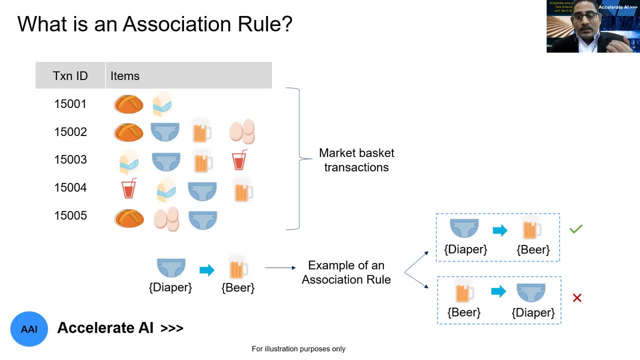 if it's, it's uh, you know the the reason? because if there is a diaper that we are purchasing, then it so may happen that we are buying beer as well, but there is no proof of if there is a beer, if there has been no diaper in that case, then we would have considered that a scenario, but that's. 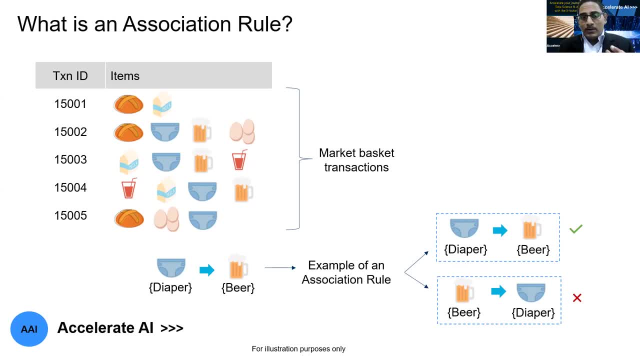 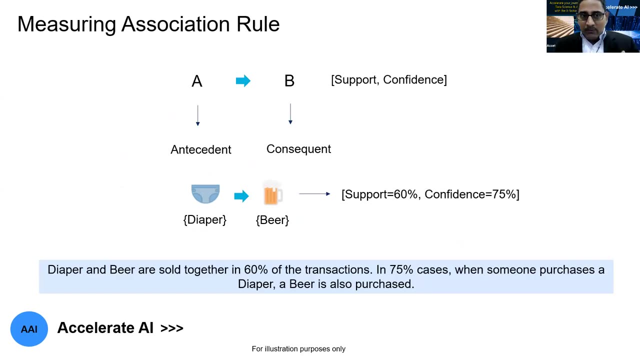 not a scenario. so hence the association rule is that if there is a diaper, then we are buying beer. so if then, if, then kind of a and distant and consequent, which is what um is. the association rule is what we say, so measuring when, when we measure this association rule, the terminology, 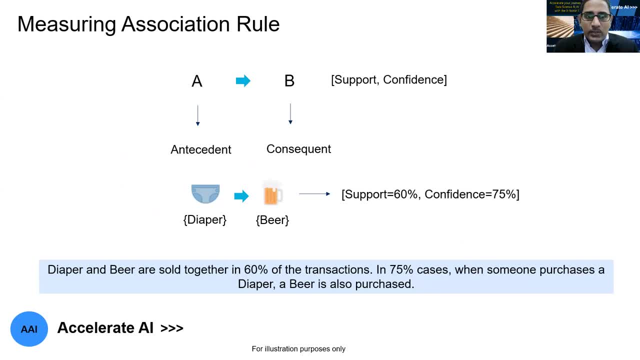 is what we are saying. if, then if part is your antecedent, which is a, b, part is your consequent, which is b. if diaper, then beer. right. so if you are buying diaper, then you are buying beer and um, there are certain measures like support and confidence here. if we look at 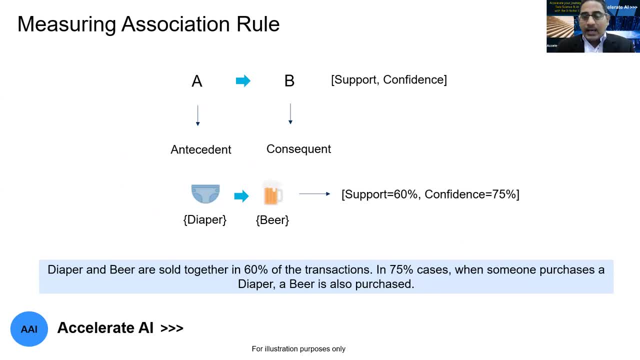 support is 60 and confidence is 75. we will see how that has been calculated shortly in the next few slides. now diaper and beer are sold together: 60 of the transactions. that's what support means. out of your five transactions: 60 of the transactions. thrice. 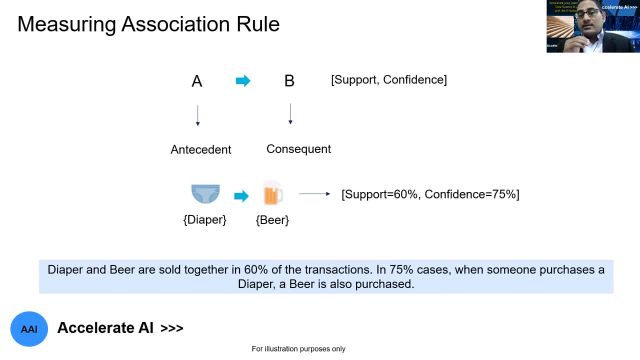 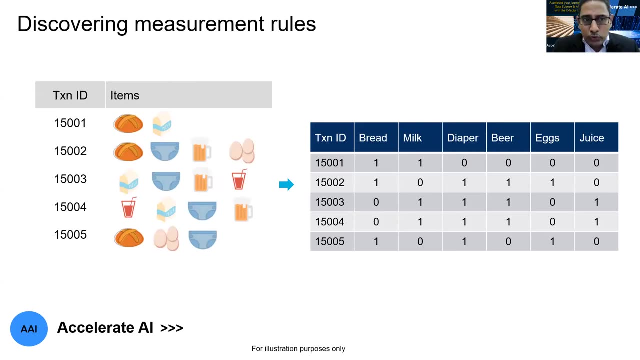 we have seen, both are sold together and in 75 of the cases when someone purchases a diaper, a beer is also purchased right. so that's the correlation. in order to discover some of these measurement rules or principles, like support, confidence and all, we have to first convert the point of sale transaction to a binary matrix format. 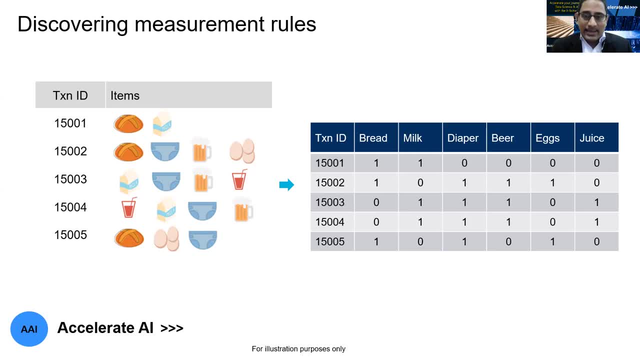 from a data representation standpoint, to analyze this, as you would see here what what we have done is we have converted this from a transaction id to the nomenclature of each of these, like bread, milk, diaper and all that, and then against each transaction id, if it exists, then there is a one, else there is zero. so we know. 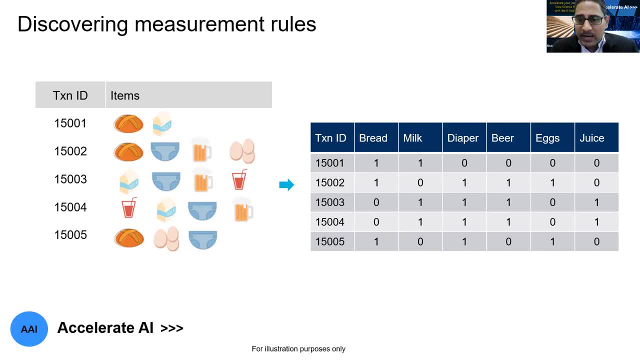 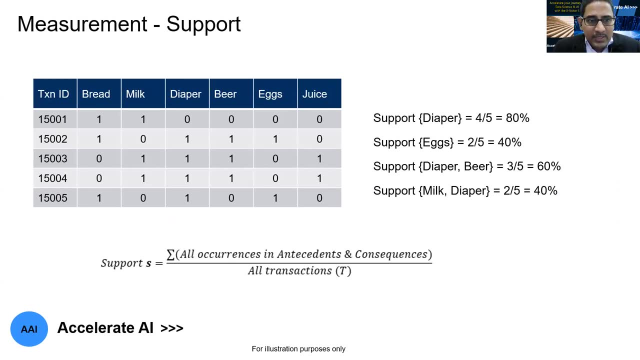 uh, very clearly the you know, kind of a conversion of this binary matrix format. you have to do that first, and then let's look at what support means. so support of diaper here means that you have all occurrences in the antecedents and consequences. so support of diaper is actually divided by all transactions. so which means you know your diaper is actually four times occurring out of the five transactions, so four by five. 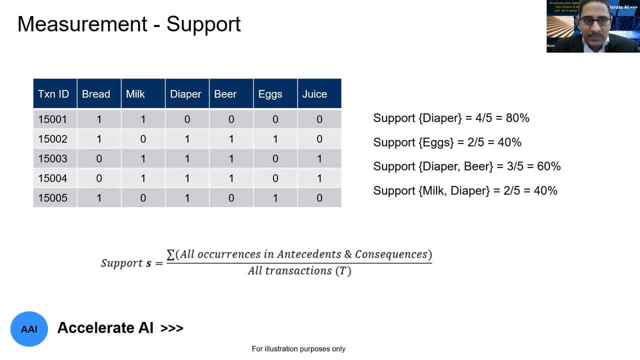 the support of diaper is 80 percent because if you look at it it's appearing in 1500: two, three, four, five. it doesn't appear in 1500 one right. similarly, support of eggs is just twice out of five, so two by five, forty percent. 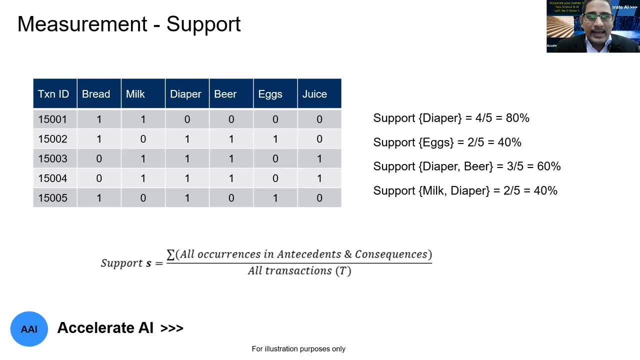 now, if we take multiple item set, let's say, say, support of diaper and beer together, if we consider both, then wherever we have both of these as one, there are three such cases where both of these are one. so the support of diaper and beer is three by five, which is sixty percent. similarly, support of milk and diaper is 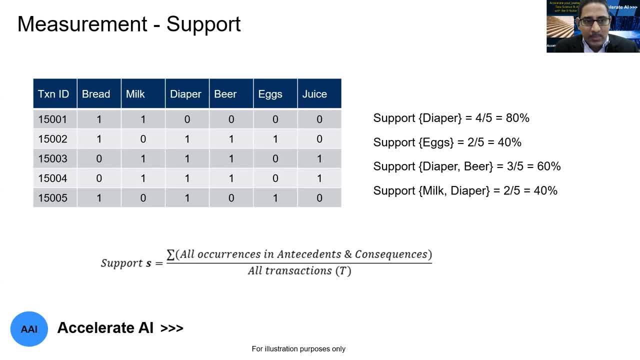 two by five, which is forty percent, because it's just appearing one. one is appearing two times two together. otherwise, one zero zero, one zero one. these are not considered here, right? so that's about the support. support is the all occurrences and distance and consequences taken together. summarization of that divided by all transactions in the database that we're considering. 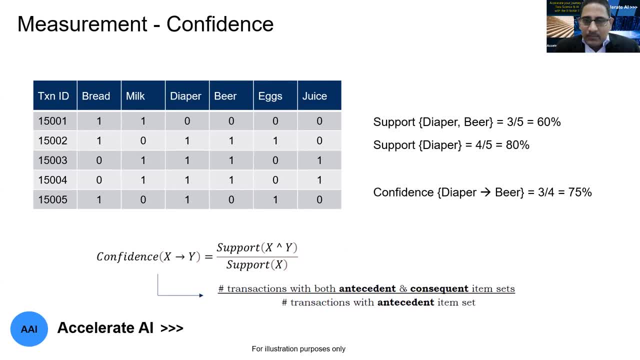 when we look at confidence, confidence is essentially, we have the support factor which is already measured. now, confidence is basically that, as a slicer, you can create a web platform to どんどんww. confidence when we say: from x to y. confidence of the fact that someone, when he or she, is buying. 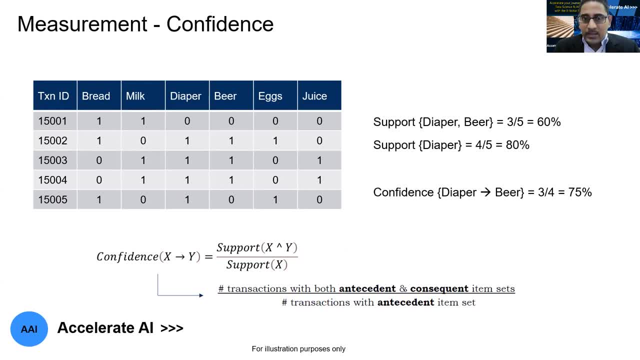 diaper, he or she will buy beer, then we we will go by the formula of support of x, intersection y divided by support of x, which means the transactions both where antecedent and consequent item sets occur, divided by the transaction with antecedent item set. now, if 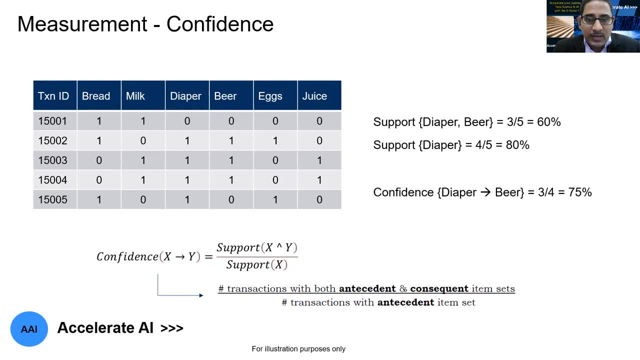 we look at that then, for support of diaper and beer is something which is diaper and beer is three times out of five, which is 60 percent, and support of diaper itself is 80 percent. so 60 percent by 80 percent, or three by four, that's 75 percent of confidence of diaper. 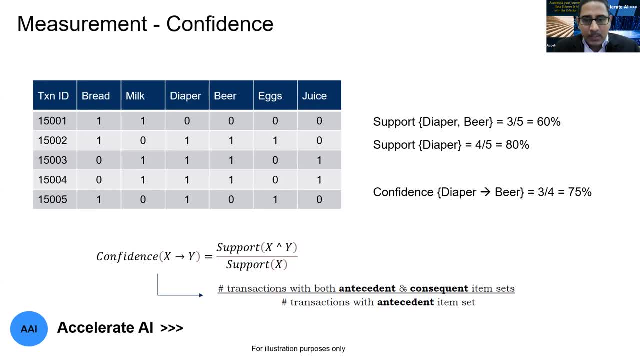 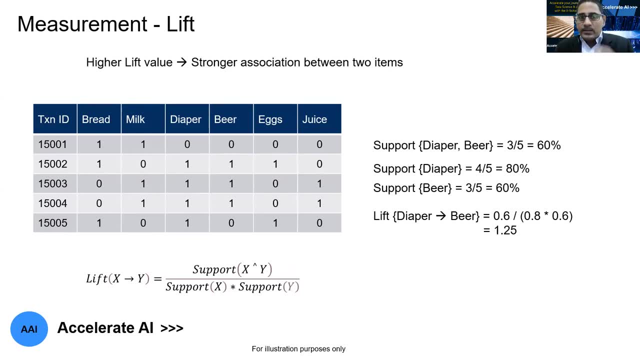 to beer, right. so that's what confidence is about when we come to lift, lift is essentially nothing but lift of x to y. it's like a support of x intersection y divided by support of x, multiplied by support of y. so here, if we look at, we have: uh, we're going to calculate the lift of diaper to beer and that's. 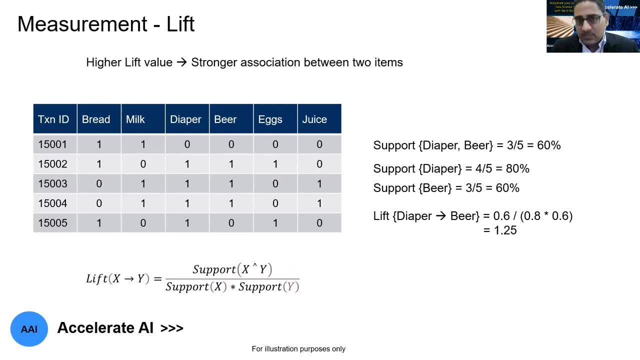 for that to happen we need to have support of diaper and beer, which is 60 percent. we have calculated earlier. support of diaper is 80 percent. support of beer is 60 percent, so it's 0.6 divided by multiplication of 0.8 into 0.6 and that comes out to 1.25. so higher the lift value, the stronger. 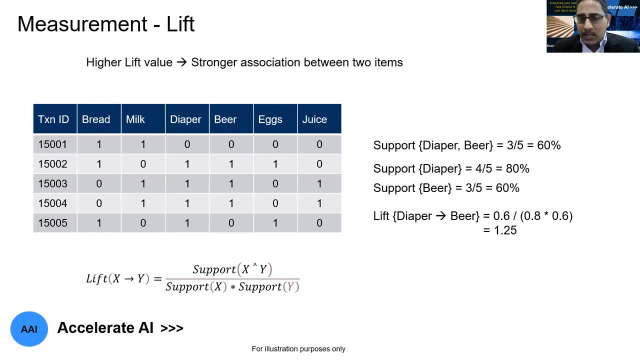 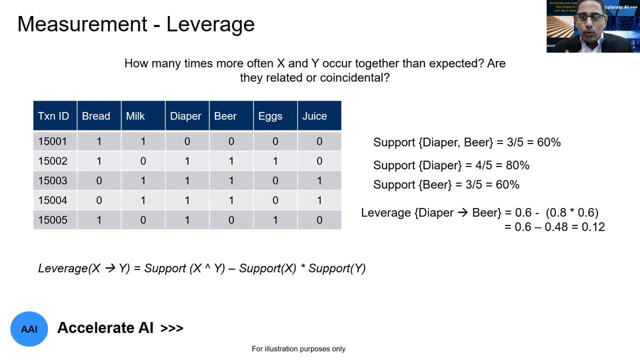 the association between two items. that's the interpretation. then there is something called leverage. leverage is nothing, but how many times more often x and y occur together than expected? are they related or coincidental? you know, that's what we're trying to. um, you know, catch from from leverage. 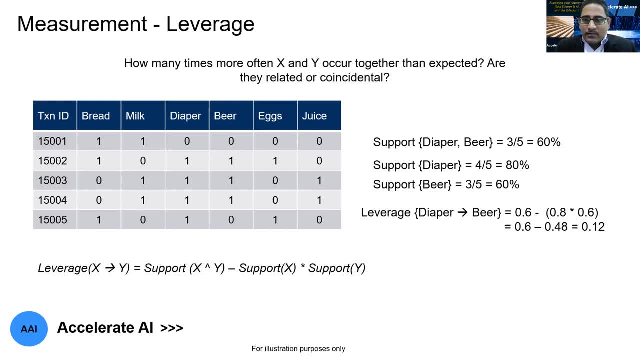 and here, similarly, considering the uh formula of x to y of leverage is nothing but support of x, intersection y minus support of x multiplied by support of y, which is where you get the value of leverage. so we have talked about the measurement factors of support, confidence, lift and leverage. 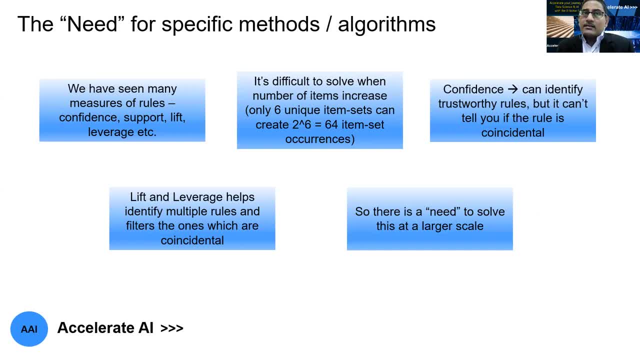 so the need for specific methods or algorithms will come into picture, because we have seen this: four different rules of measures, right, or measures of rules. now it's it's difficult to solve when the items increase because we have seen six item sets, unique item sets and it could. 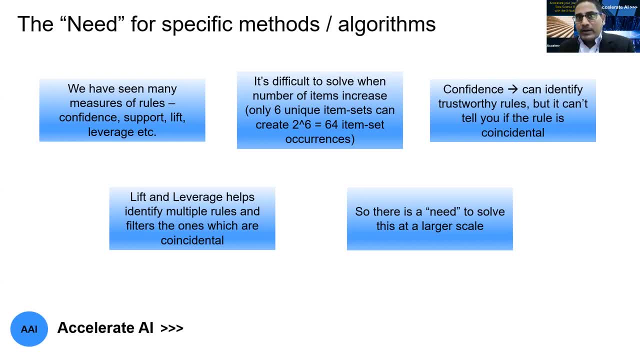 create 64 item set occurrences and of course you have to find out the frequent occurrence of the item set and so on. so the the problem is when it is so large we can't really go and manually solve it, so hence we would need algorithm to solve this complex. 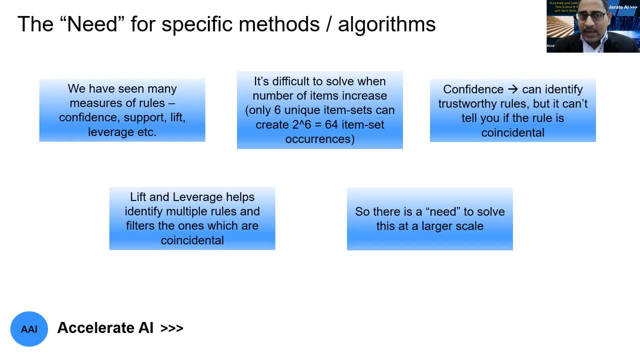 problem. there is a need to solve this at a larger scale. that's why we we have that. and another aspect is when we look at something like confidence. it can identify trustworthy rules, but it cannot tell you if the rule is coincidental, so we need to understand where it is related, where it is. 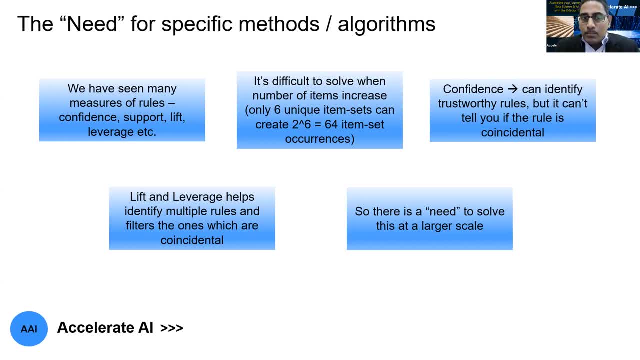 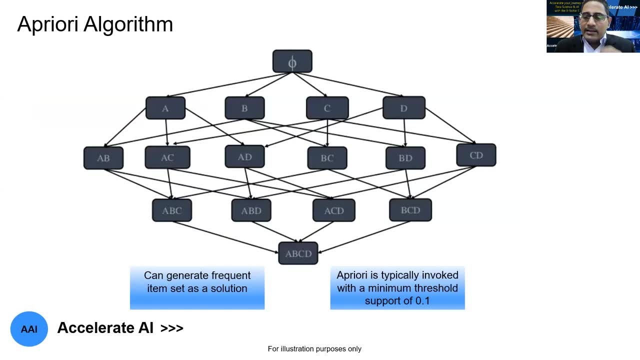 coincidental. so from from all the factors, it's it's important to go into an algorithm, and that's where we we can't really go and manually solve it. so hence we would need algorithm to solve this complex problem. we get into something called as a priori algorithm. it's an algorithm for frequent item set mining. 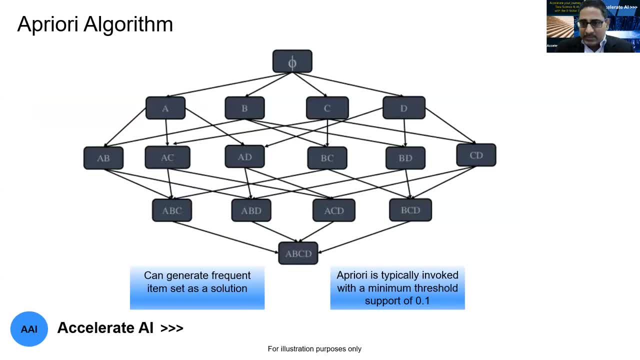 and association, true learning over relational databases. it. it proceeds by identifying the frequent individual items in the database and extending them to a larger and larger item sets, as long as those items appear sufficiently often in the database. you know, that's why we use a priori algorithm and if you you could see that the frequent item sets determined by a priori can be. 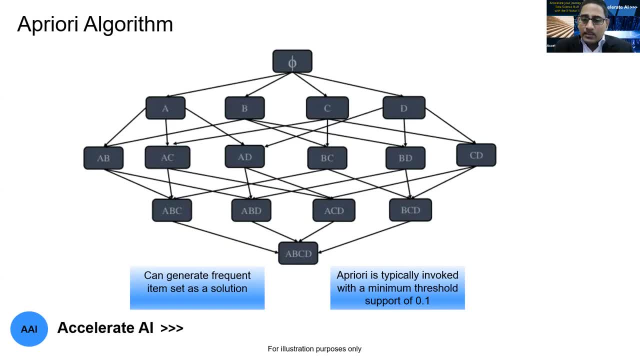 used to determine association rules which highlight general trends in the database. you know, and this has applications in domains such as market basket analysis and so on. and here, if we look at the algorithm or at a high level view of it, you would see we have considered four items: a, b, c, d. so to 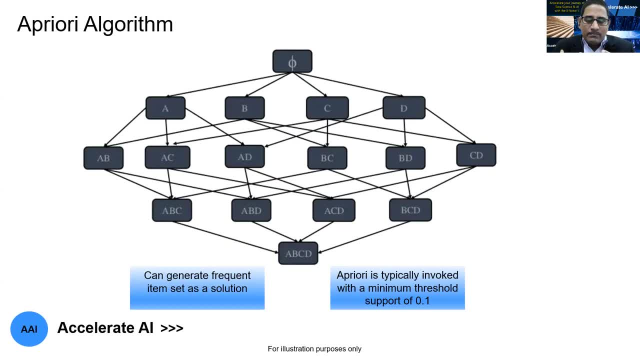 start off with the way it works. it generates k item sets, um, you know, as part of it for k products, first it sets the minimum support criteria, then it generates a list of one item sets that meet the support criteria. so it starts with null. then you know identify a, b, c, d. 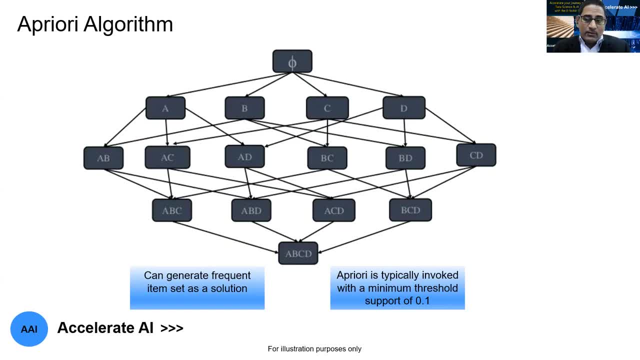 individual items and then it use the list of one item sets to generate the list of two item sets. so, for example, i have a. it will start getting a, b a, c, a, d right. similarly, for b a b is already there, so you know it could be b a b. 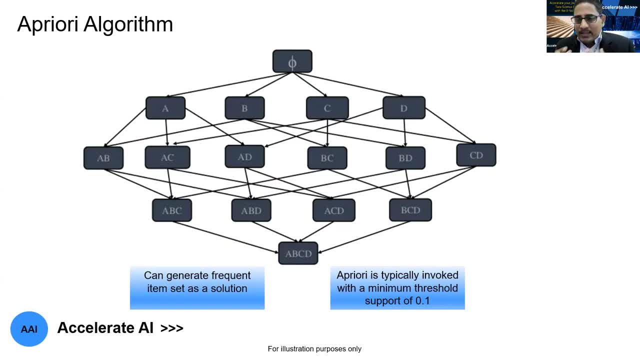 already there. so bc bd, that's all right. so that's how it gets created. then it uses the two- uh, list- of two item sets to generate list of three item sets. it could be uses a b to go for a b, c, a, b, b, because that's where a, b is involved, but c and d are the other item sets and so on. right, and then 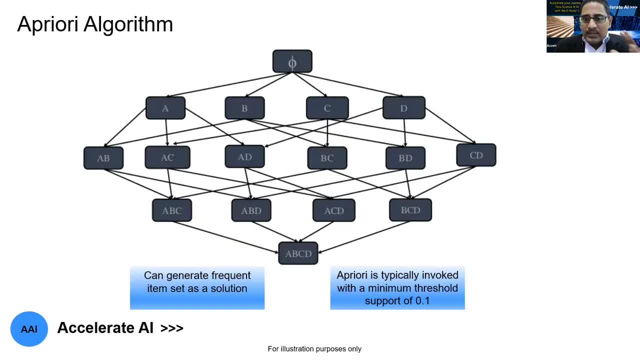 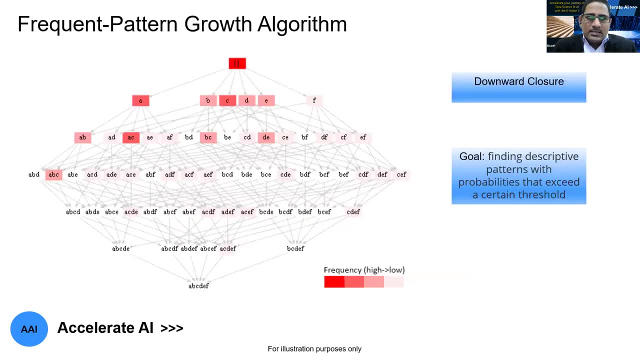 of course. last one is a, b, c, d, where it's only one. so that's the, that's how it continues up through the k item sets and it creates and a priori typically invoked with a minimum threshold support of 0.1, but that that can be used appropriately. uh, similarly, there are other. 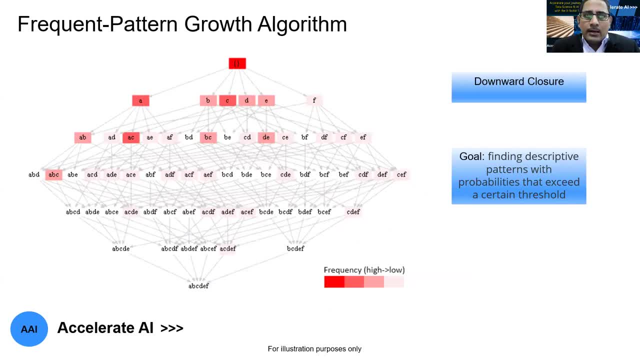 algorithms. we will not go deep into it. but frequent pattern, uh, growth algorithm is um, the. the intuition here is, you know, frequency can never increase. when we add a new item, it can only decrease. so this is called the downward closer, and that's where um the the objective of finding 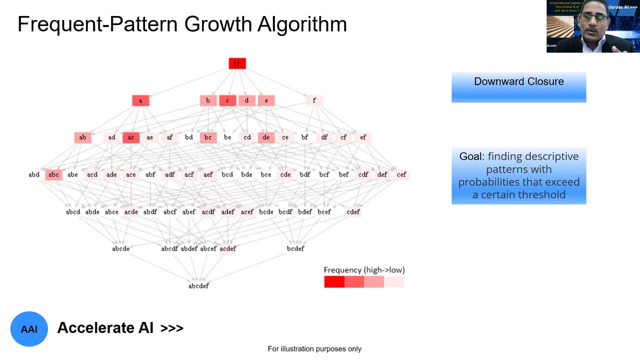 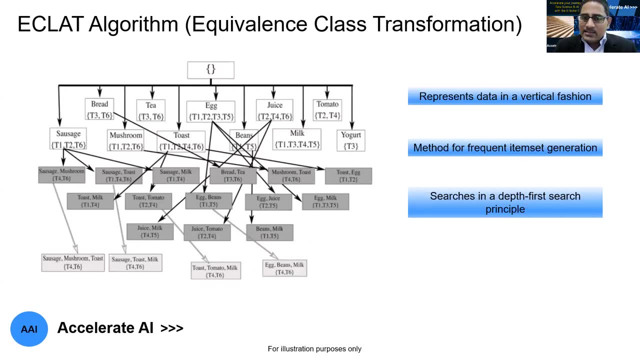 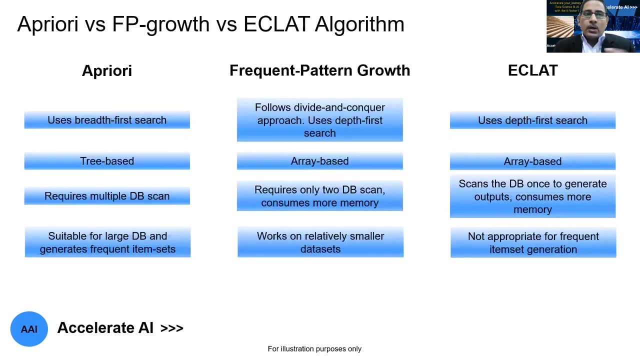 the script patterns with probabilities that exceed a certain threshold is where we use frequent pattern algorithms. similarly, there is something called as equivalence class transformation. it represents data in a very vertical fashion. it's slightly different. it searches in a depth. first search principle approach and this is another algorithm as well. so if you look at um, you know a priori. 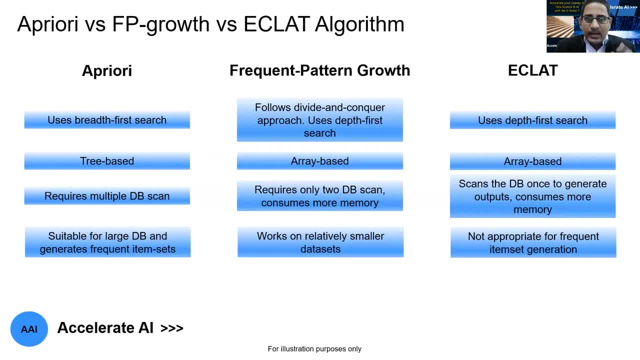 fp growth and um ecl t. all of these three a priori, is something which uses the bread first search. uh, it is tree based, it requires multiple database scan and it is suitable for last databases and generate the frequent item sets. that's, that's how the principle it and then others are slightly different than that. 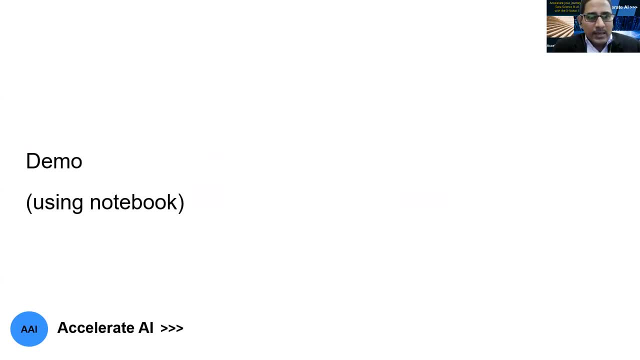 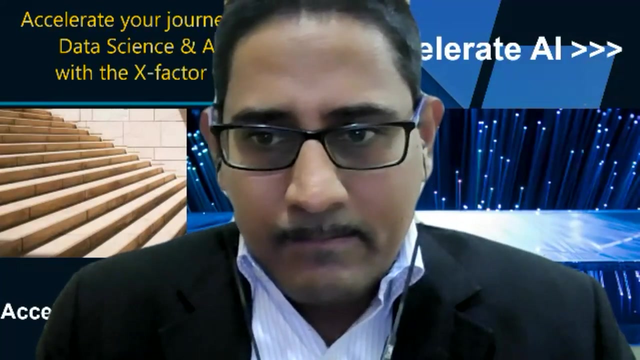 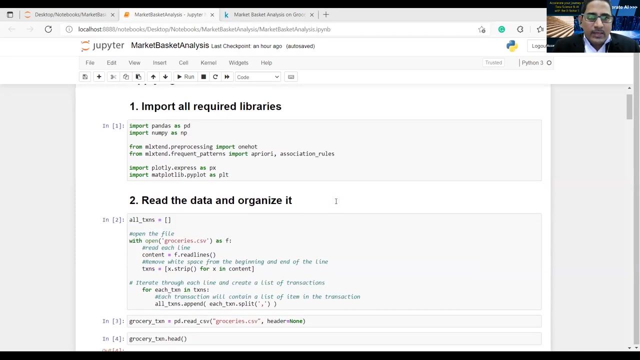 so let's get on to um the the demo using um the notebook. we will jump on to um the the notebook now. next we will see at the top select買는 and select buy our statement. okay, so hope um you're able to see this when we start looking into the the notebook. what we 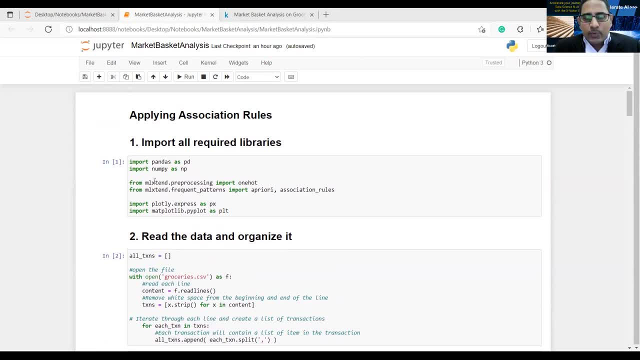 typically do is we import all required libraries. um, we have considered a groceries data set for market basket analysis. this is possible because we basically need these uh main mission database funnels- market basket analysis- as part of this example. This is available in Kegel and other places. 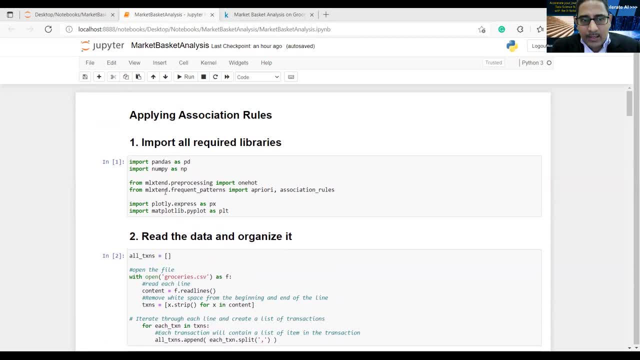 What we need to do is what we have done. here is something like ML extend package very specifically used for market basket analysis And we are using for pre-processing. we're importing one HUD And for the frequent patterns from ML extend, we're importing a priori and association rules. 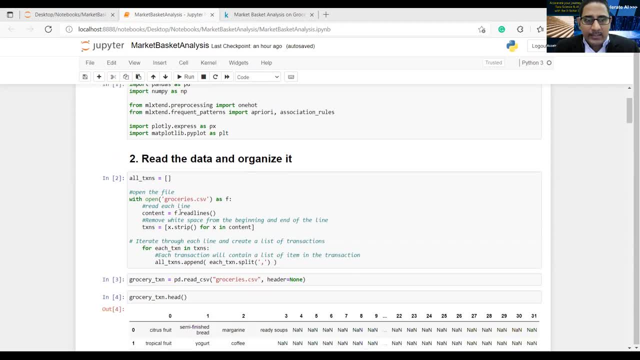 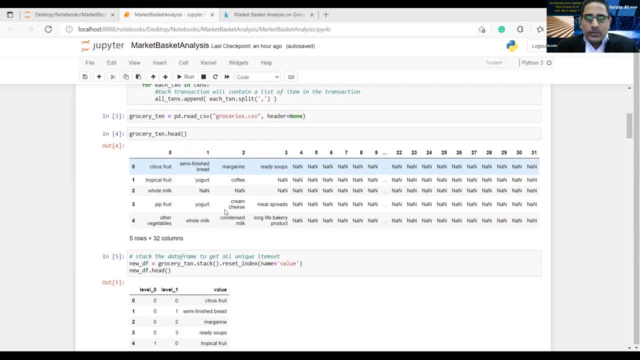 And then, of course, some of the data visualization related stuff, and then NumPy and Pandas. So we have read the data and organizing it. When we start reading it from the CSV file, we could see there are different type of elements like citrus fruit, tropical fruit, whole milk. 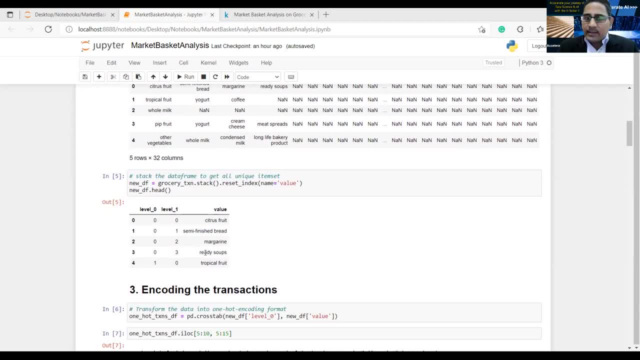 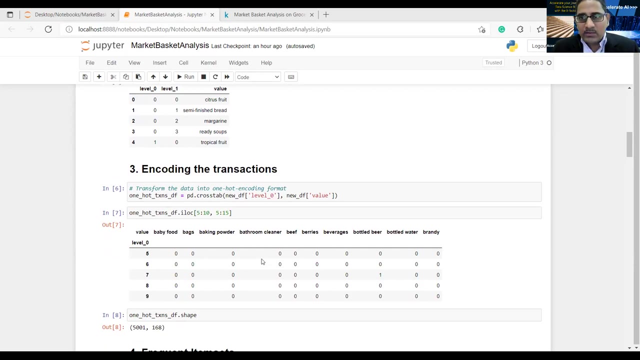 all of these things that we have. Then we would like to stack the data frame to get all unique item sets by value, So it does a presentation in such a way that we have the values like this represented and then we encode them to a transaction. 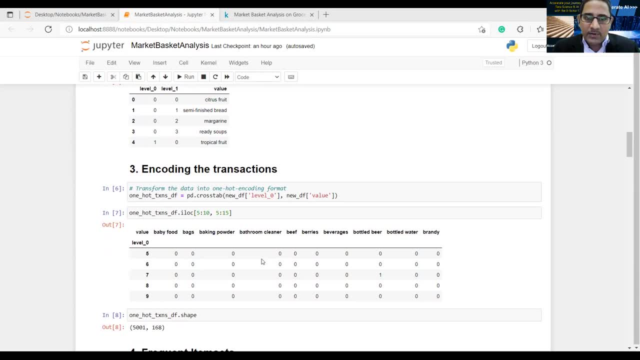 because we've seen, from a point of sale to a binary, kind of a format where we want to have all of these one HUD transactions, kind of a cross tab where for each of the row item we have the value or the name of the item. 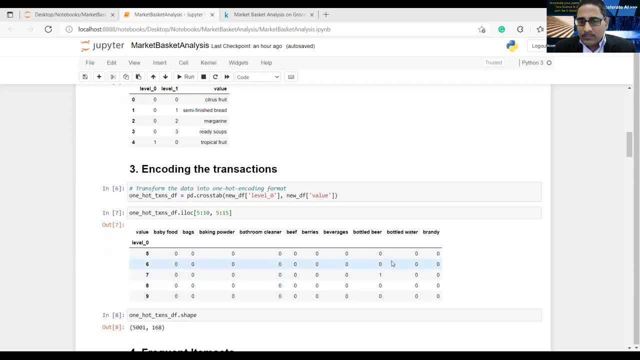 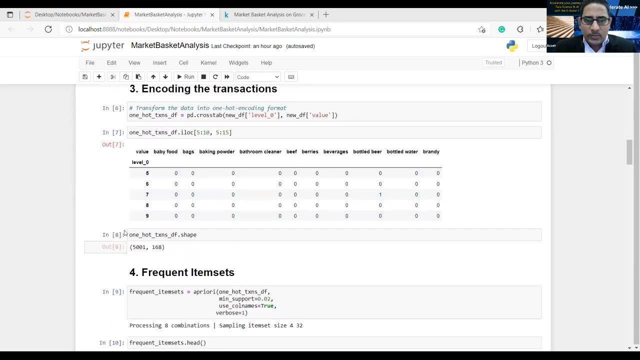 like baby food bags, baking powder, and then the binary value of it, whether it is existing as part of that transaction item. So here, as you would see, as a sample data set, we have kind of 5,001 rows and 168 such columns that we have. 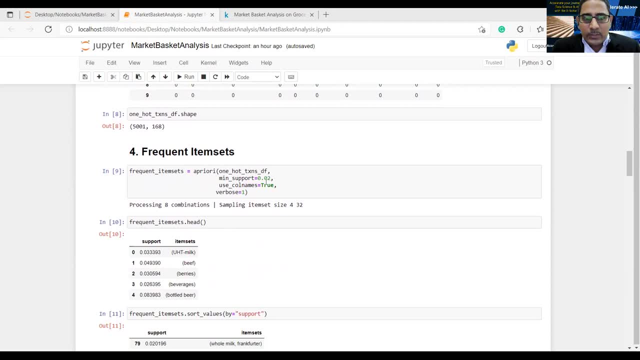 Then when we try to capture the frequent item sets, we will use a priori the data frame that we have. Then we have used a minimum support of 0.02, and you can use column names too, And then for both one we'll show you this. 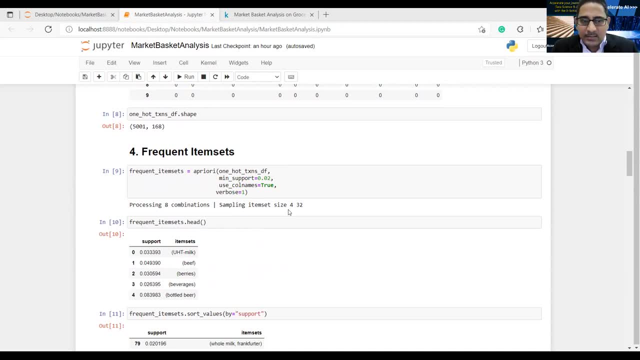 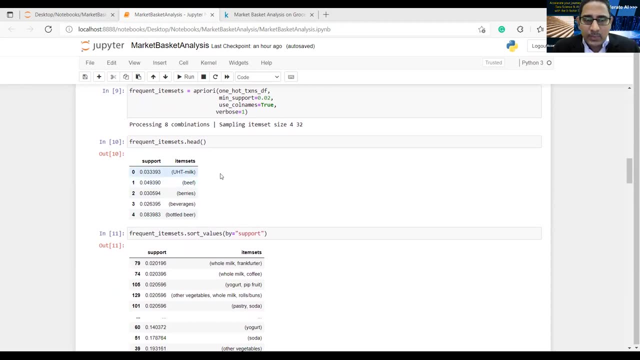 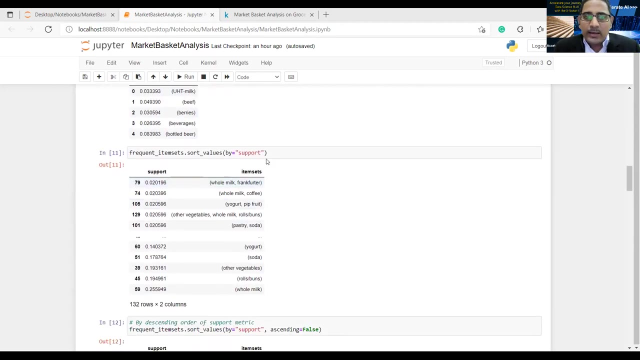 processing how many combinations and what is the sampling item set size which shows that. And then when we do initial few rows of the frequent item set with the support value, it shows us the item set and the support of it. Then we sort the values by support. 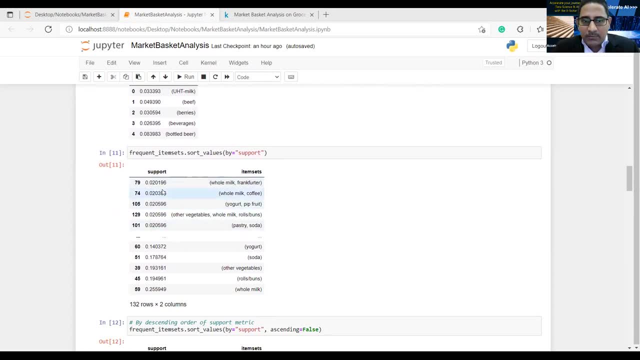 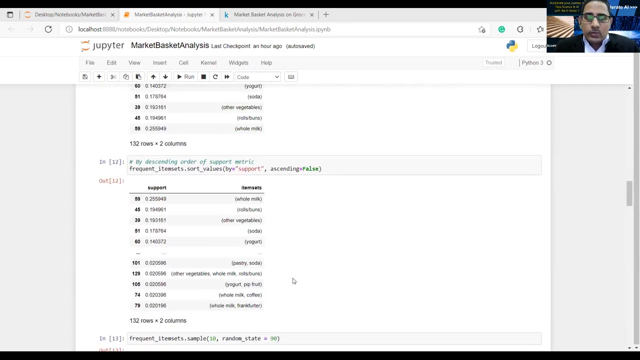 Then we get that based on the support value. what are the item sets are attached to it. So in this case, let's say whole milk and frankfurter is something with 0.020196 and then so on. Then we try to get the support, the frequent item sets. 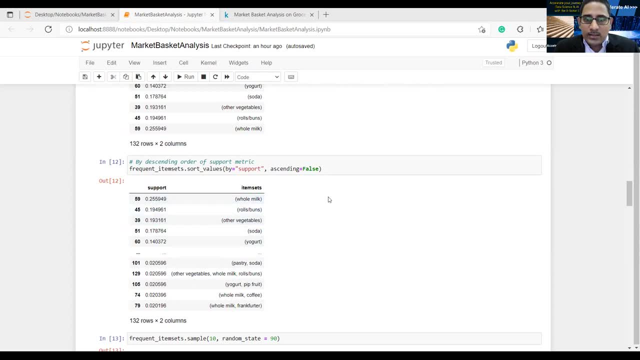 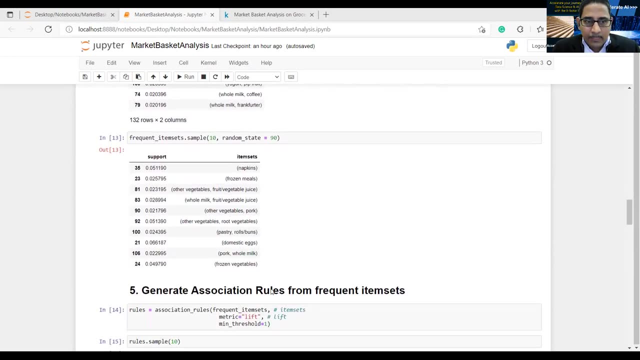 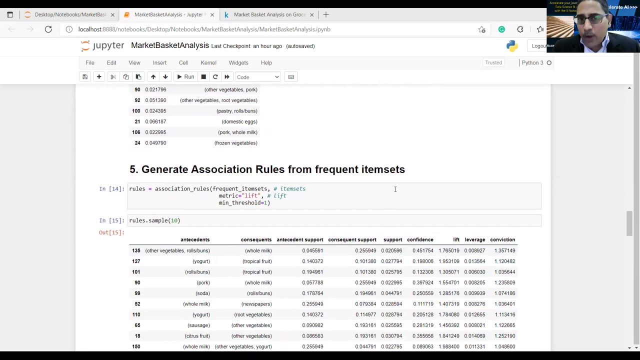 We sort the values by support and in an ascending order, so that the whole milk is having the highest support And then it follows by that. So then we use kind of generating the association rules from this frequent item sets. Now we have the frequent item set. 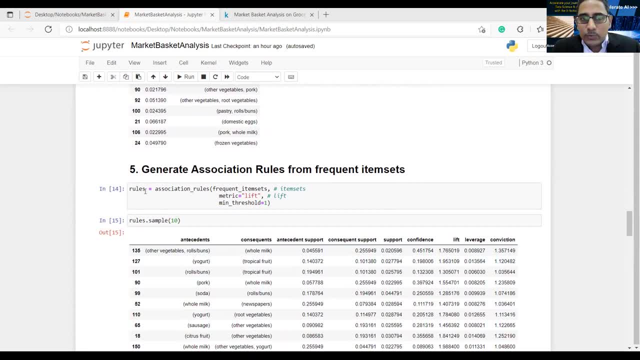 which is created and is available with us. Then we'll use the rules, where we'll use the function association underscore rules, And then we take the item sets, the frequent item sets. Then we say what metric that we are going to use. 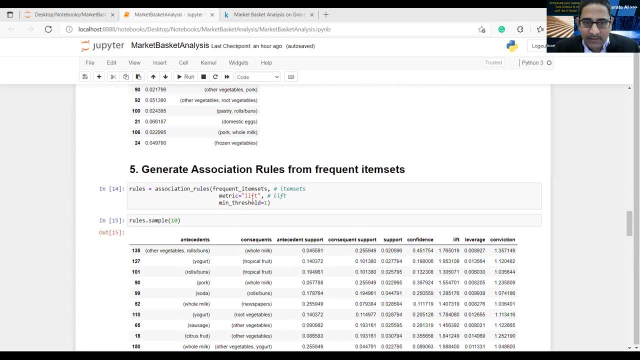 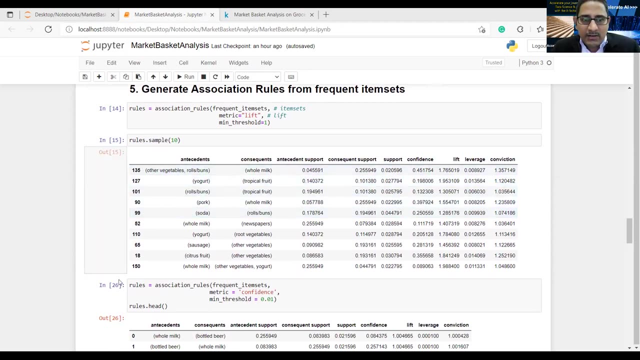 Is it lift? Is it something else? So we are using lift here with a minimum threshold of one. We don't want anything which is below one, We just want everything which is above one, so that we get those item sets. And that will give a kind of a sample of top 10 records. 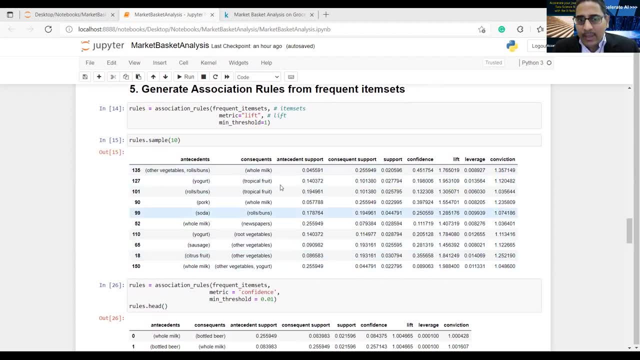 where we see Antiss Stephen's consequent. So this is your A then B. if A, then B, right, If you're buying yogurt, then you're also buying tropical fruit, that type of thing, And then for each of these you have a Antis Stephen support. 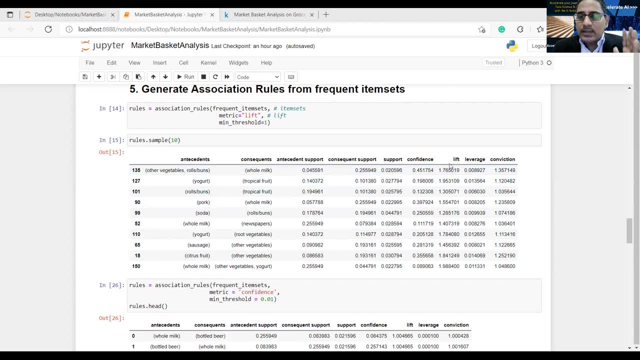 you have a consequent support, you have a overall support, then confidence, then lift, then leverage. There's also something called conviction. So there are a lot of these parameters, so the majors are kind of represented as part of association rules when we use this. 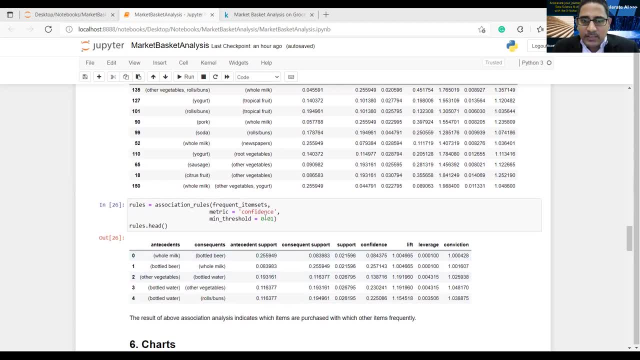 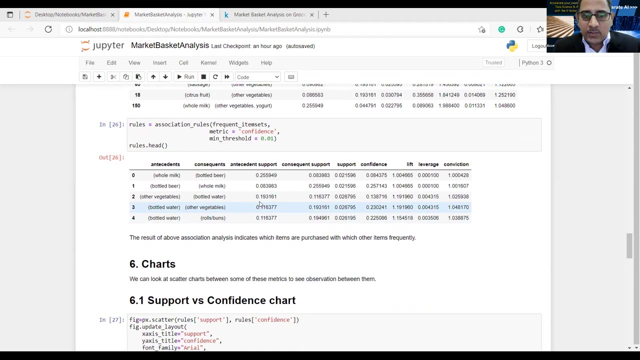 then we can always change the metric to confidence and set the threshold whatever we want and based on that it will show accordingly. so we can play with the same data with a different metric and a certain minimum threshold, and we can. the result of that association analysis will will indicate: 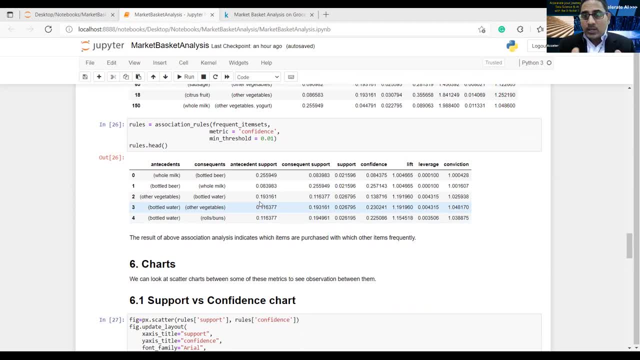 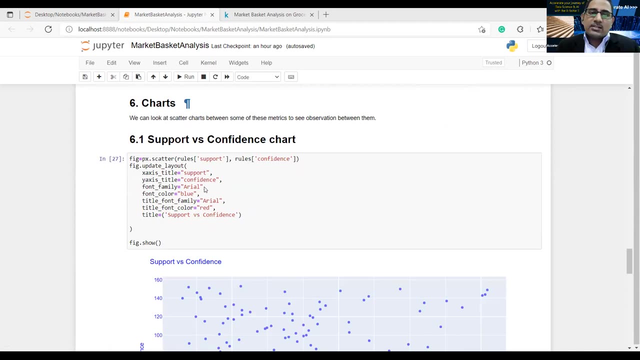 which items are purchased, with which other items frequently and of course with with higher support or higher confidence or higher lift and all that stuff that we can measure accordingly and represent. in this view, we can also do a chart, kind of a scatter plot, between these metrics, like: 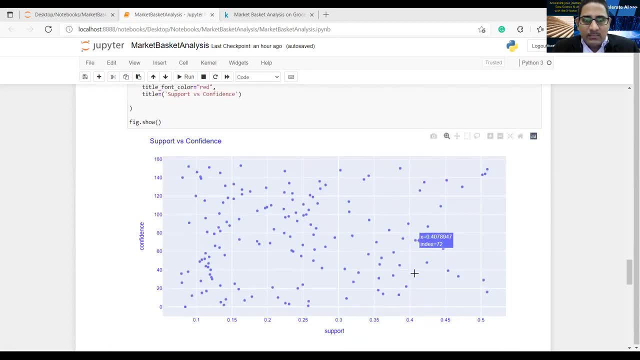 support and confidence. when we plot that, you know, we see the values of support and confidence and here are some of the metrics that we can measure. and we can also do a chart, kind of a scatter plot, of these items with with the x and the index values there. so you'll have an understanding. 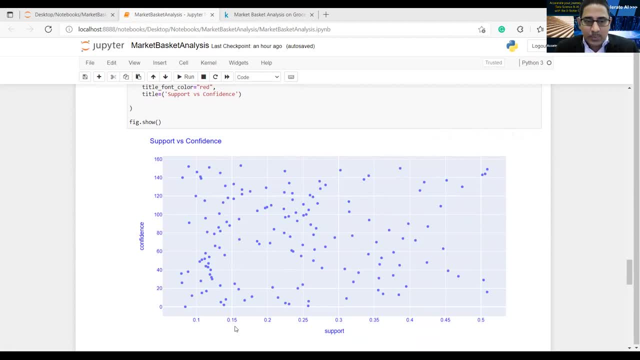 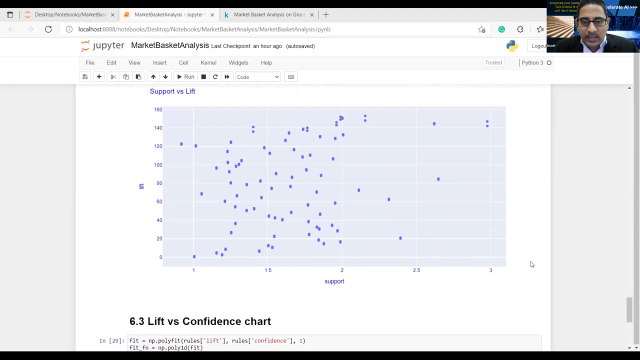 of how many item sets that we are looking at. if 0.15 is the support and 60 is the confidence, 60 is the confidence, then then you know we are looking at. you know something like this right? so similarly we can also look at the support versus lift. so this is support in. 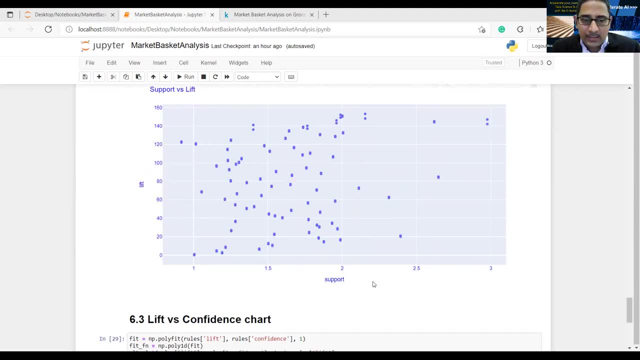 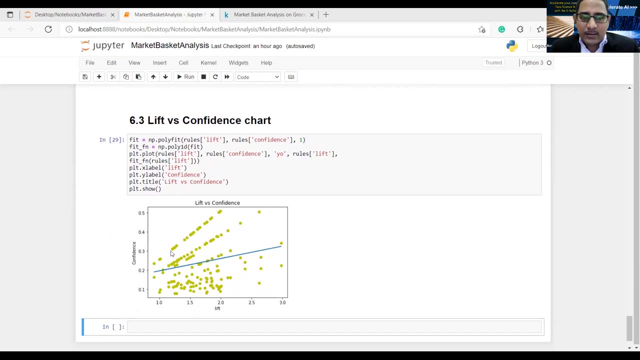 x-axis and lift and y-axis and accordingly we can look at that similarly, lift versus lift, and this gives us this confidence also that we can look at it and that will give you know this is again a representation of kind of a polynomial, you know, representation of line, to see how it is. 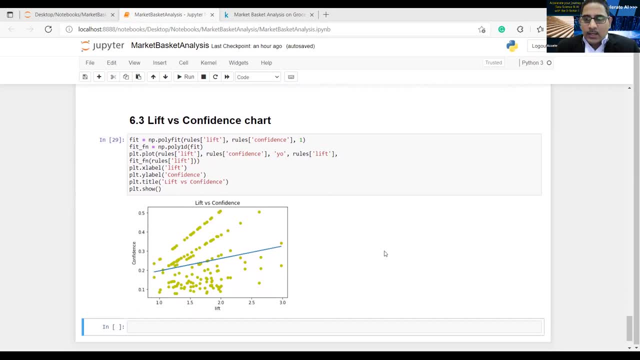 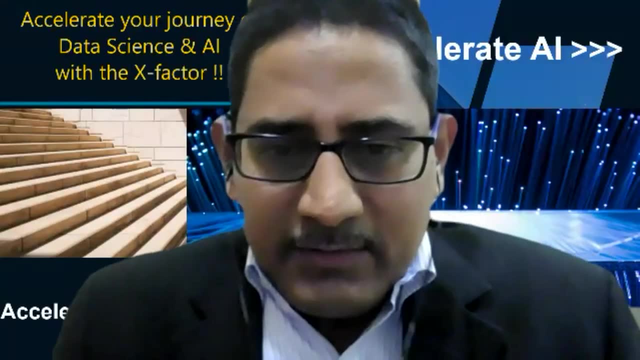 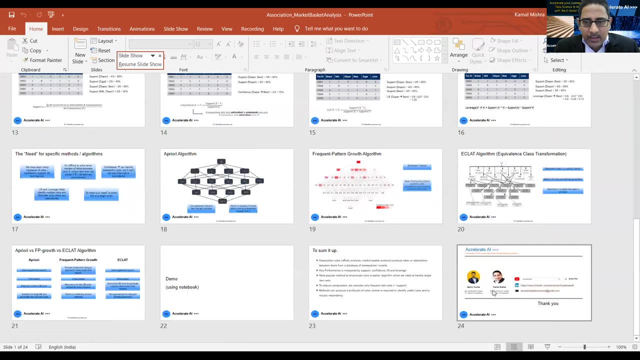 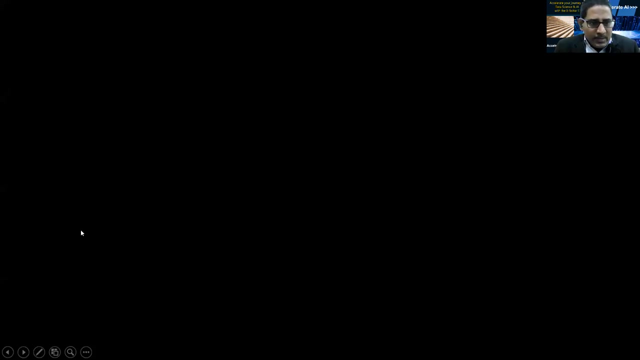 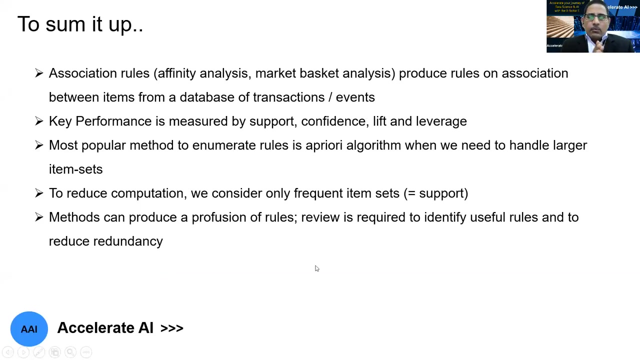 represented the values across these two as a scatter plot. so that's about it, and so we have covered. let me quickly take you through to the summary portion of it. And yeah, so, let me just a minute. Yeah, So what we have looked into it is: